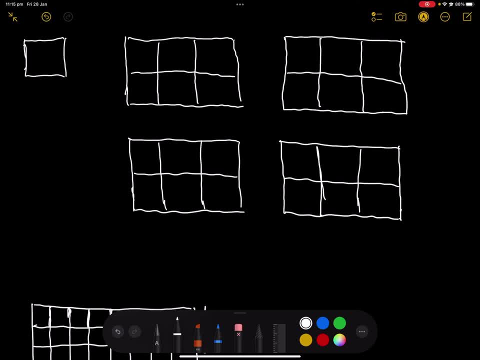 Okay, let's have a look at the first square I drew. It's made by four sides, two horizontal and the two vertical. So let's make these two horizontal and two vertical and two horizontal. So four sides makes one square one. 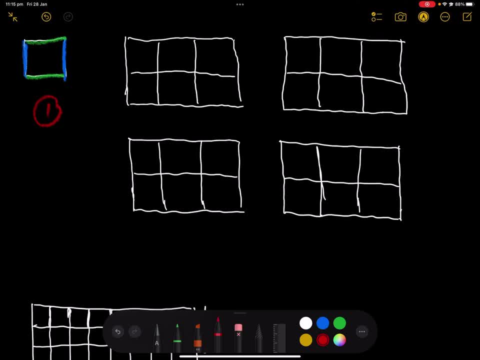 Okay, second one: We have three horizontal lines and four vertical lines. If I choose different horizontal lines and the different vertical lines, you will see we make different size of the square or rectangle or on the different position of the square rectangle. So if I pick these two vertical lines, for example this one and this one, 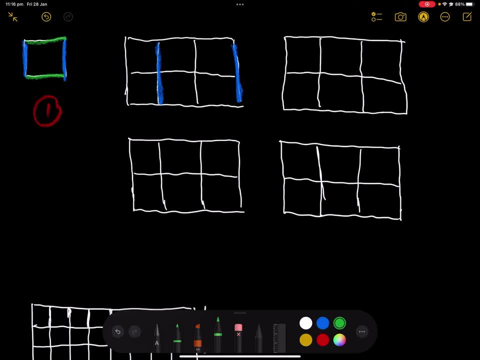 and if I pick these two horizontal lines, this one and this one, then you will see I made this rectangle. But if I choose different one, different horizontal and different vertical lines, you will see I make different square. Let's see if I'm making these two still are vertical. 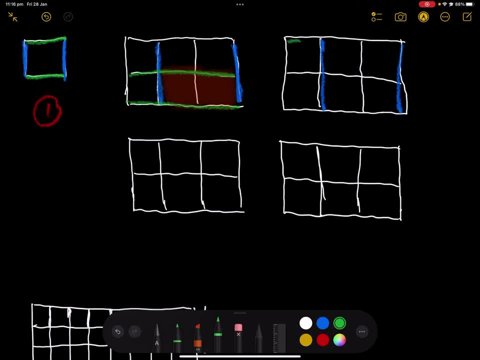 but if I change the horizontal into this one and this one, then you will see I actually made these squares bigger- one right. And if I change the vertical ones into this one and this one and I change the horizontal one into here. 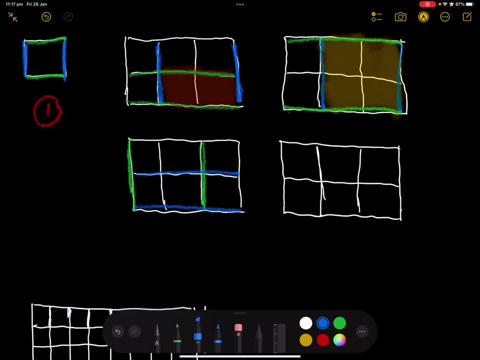 and here I made the same size of the rectangle as the first one, but different position this time And then again. if I change mine again with vertical line is these two and the horizontal line is these two, then I actually made a biggest. 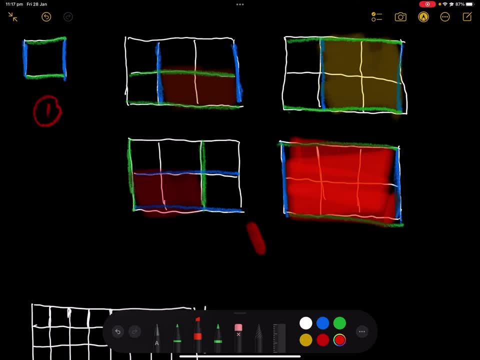 rectangle, Right, okay, So with all these different choices of horizontal, vertical line, I can make all these different sorts of the square and the rectangle. So how many choices I have in this shape? I made four vertical lines and three horizontal lines. So for vertical line I have: